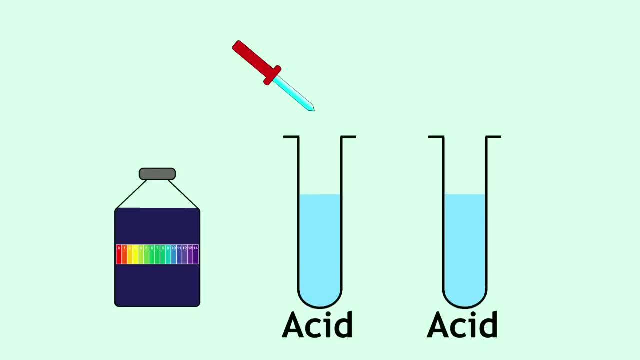 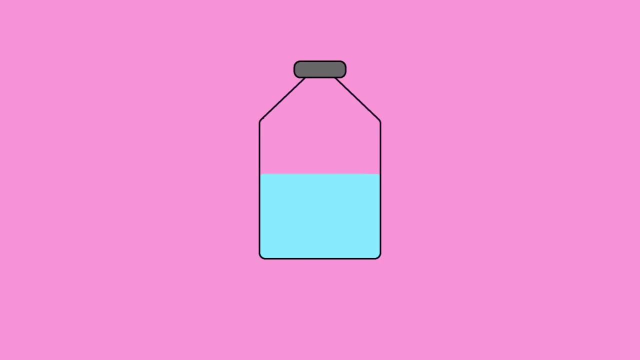 We can test for acids using universal indicator solution or paper which turns red or orange, all depending on the strength of the acid. Blue litmus paper also turns red in the presence of an acid. An example of an acid that you are likely familiar with is hydrochloric acid. 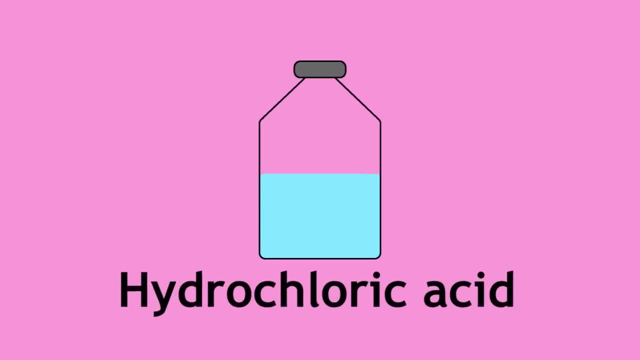 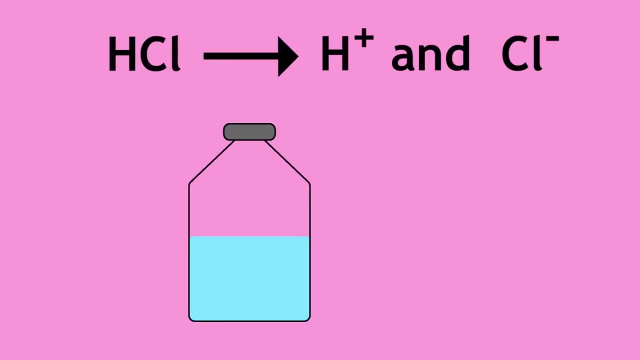 Hydrogen chloride dissolves in water to give hydrochloric acid. Hydrogen chloride will dissociate to give a proton and a chloride ion. The proton is not just released, but it is transferred to another substance. For our example, water accepts the proton to form a hydronium ion. 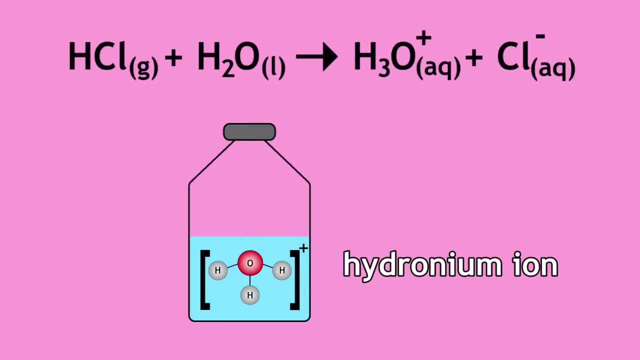 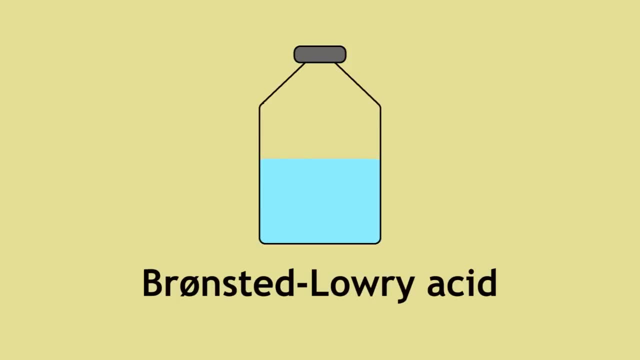 A hydronium ion is also known as an oxonium ion. A Bronsted-Lowry acid is a substance that releases or donates protons in solution, in our case, hydrogen chloride. A Bronsted-Lowry base is a substance that accepts protons in solutions. in our case, 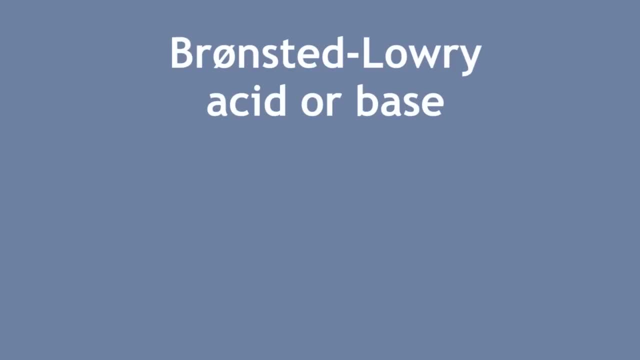 water. Notice that the definition of a Bronsted-Lowry acid or base is not a function of pH. So an acid-base reaction according to the Bronsted-Lowry theory involves the transfer of a proton from one substance to another. 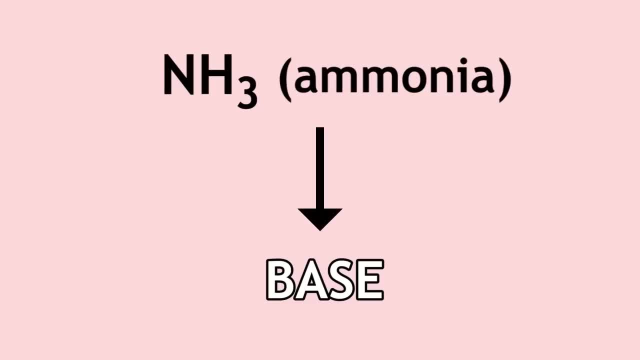 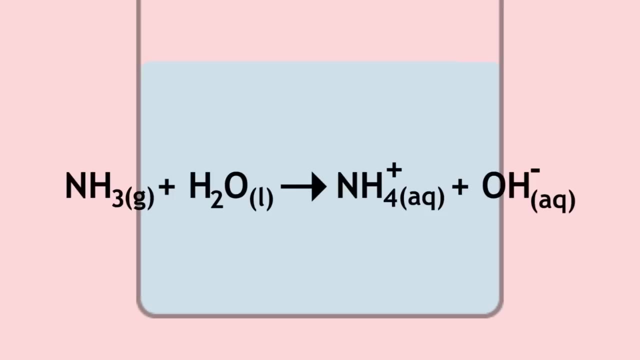 In the introduction, we mentioned that ammonia acts as a base, even though it does not release hydroxide ions, which is stipulated in the Arrhenius theory. When ammonia dissolves in water, it accepts a proton from water. Notice that this reaction also involves a proton transfer. 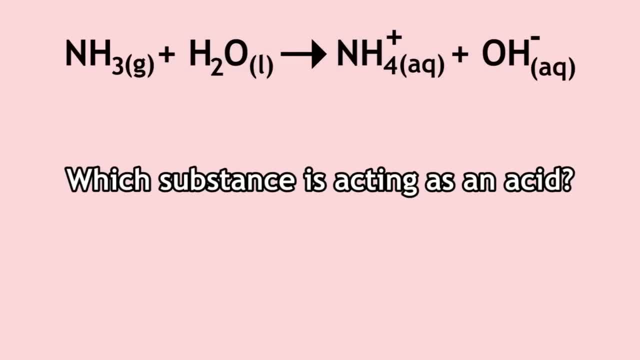 Can you figure out which substance is acting as an acid in this example, Which is acting as a base? Please pause the lesson to think about this and resume when you are ready. In this example, water acts as a Bronsted-Lowry acid because it releases a proton. 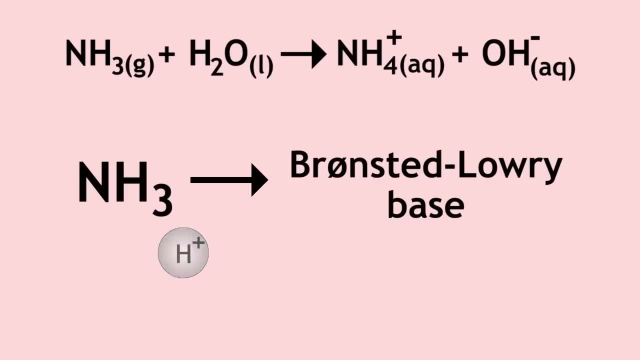 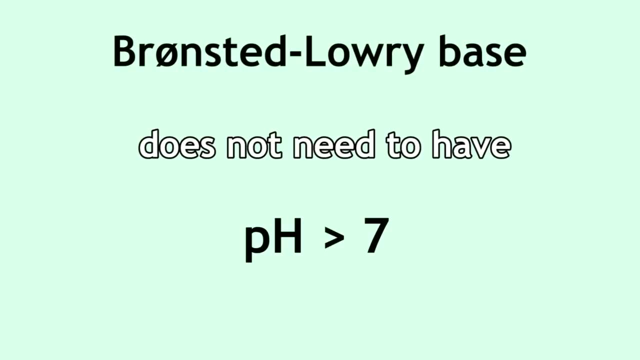 Ammonia acts as a Bronsted-Lowry base because it accepts a proton, So a base according to the Bronsted-Lowry theory does not need to have a pH greater than 7, or turn red litmus paper, blue or turn universal indicator solution or paper.